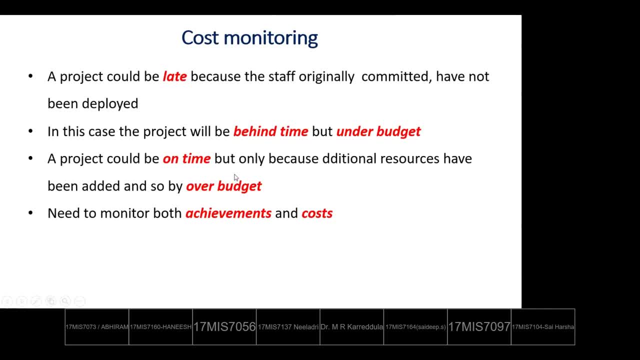 Of course it is in under budget only The project could be on time, but only because additional resources have been added and so by over budget. So Here, if you add the resources, That is, human resources, software resources, hardware resources and various other environment factors that are required to finish the product, 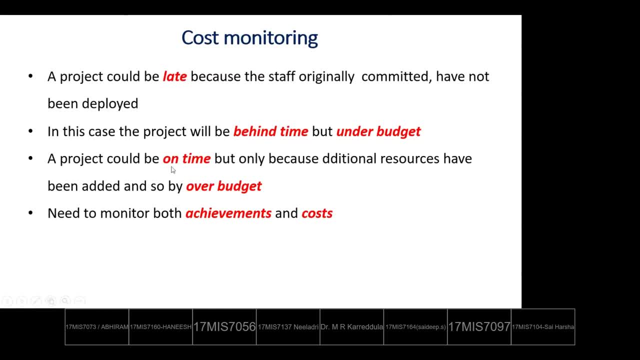 If you add these resources on time, we can easily finish it. If not, if you add the resources at lately. so that is a later stages of the development, That is, during testing or maintenance, or sometimes we are trying to adding during deploying. 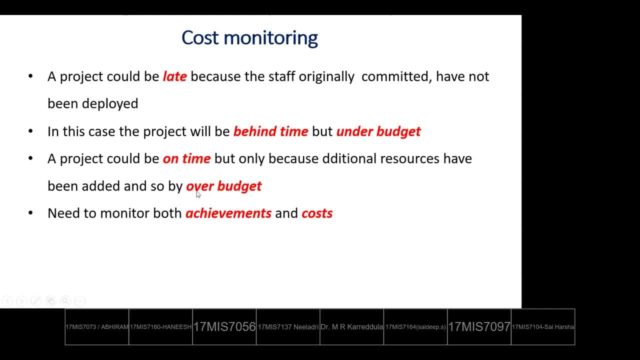 So Okay, It leads to our budget, So we need to identify the right number of human resources at the time of commitment and, deploying the same number If possible, deploy more than the identified. Then we will deliver the product by the given deadline to the client. 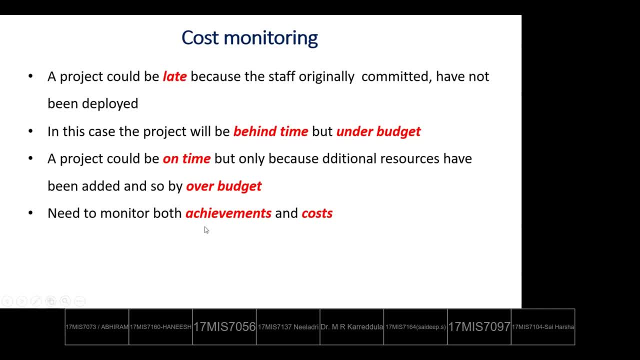 Need to monitor both achievements and costs. Achievements- what During development, from top to bottom. The initial problem is divided into various modules. Okay, All modules are divided into further sub modules. sub modules into lower level elements, objects and their costs during development. 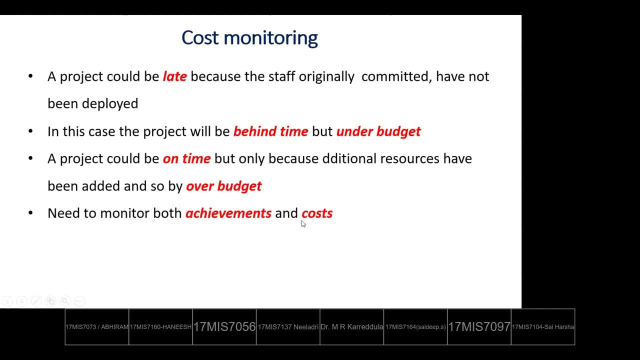 What is the cost of the object and task and parent task, grandparent task and so on, And how many are scheduled for this week, for this month? How many are achieved? So what do you mean that achieved finished by the given deadline? What is the cost applied or implemented on the achieved task? 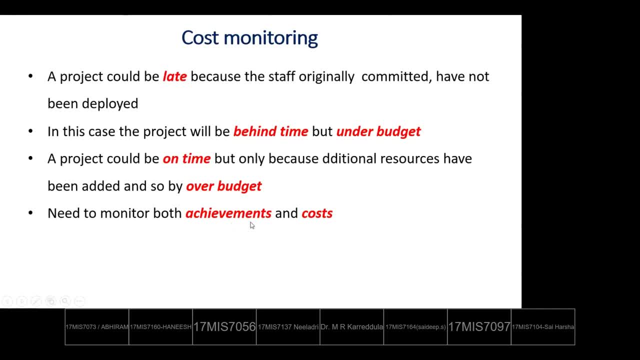 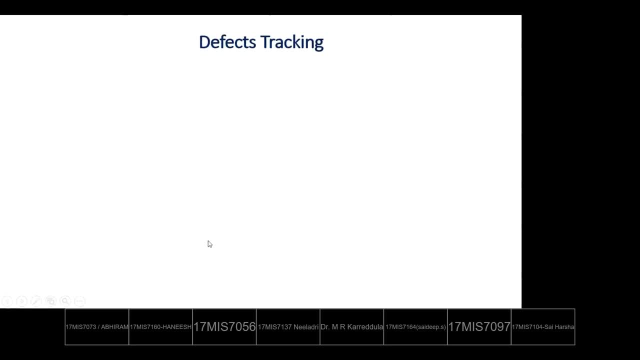 So we need to monitor these things So that we will discuss furtherly in allocation of resources in the next session. So this is about cost monitoring, Then defects tracking, So during development various defects are identified. It's not same like as an error. 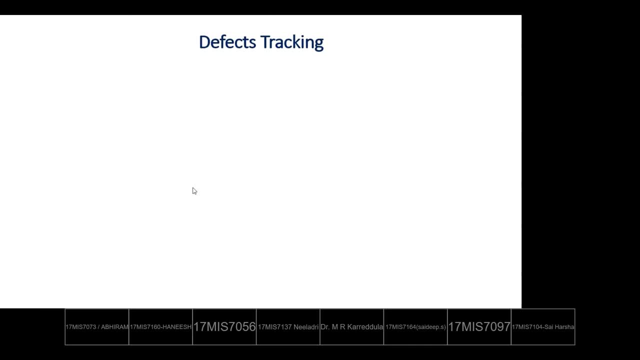 So what do you mean defect? Why defects are occurring during development, We'll see. So defects can occur at any stage in software development cycle due to mainly to human error. So defects are occurred because of human error. So that is, the various human resources are involving in terms of analyst, designer or architect, or developers, group of developers. 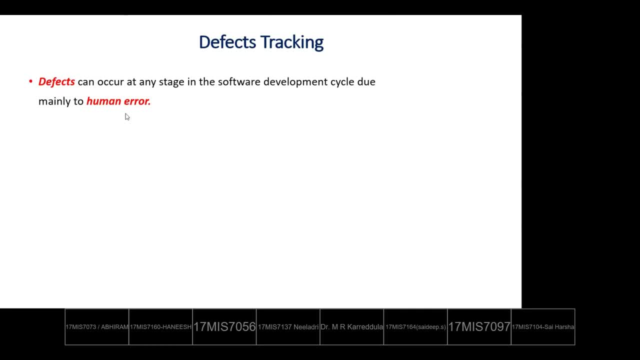 Probably hundreds of thousands, are working Test engineers, maintenance engineers, content writers, etc. etc. So here, due to the human errors, these defects are happening during the project schedule, also in development of the project, Why humans are doing mistakes. So what is the first step in software development? 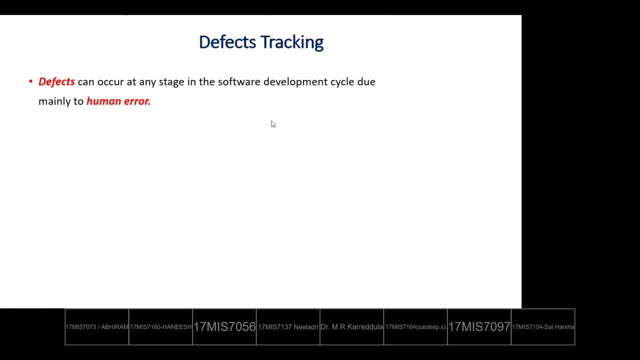 Defining the problem. So, prior to define the problem, collecting the requirements from the client, That is, customer communication. Collecting the requirements from the client. So, in order to collect the requirements from the client, we will use, generally, the globally accepted language. 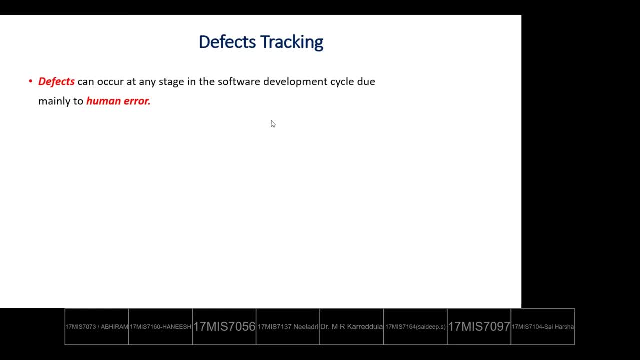 What is the language? English? English language is used to define the problem. So the greatest flexibility or advantage or disadvantage of English, like language, is: we can understand our own way, The others can understand their own way. So one thing may be conveyed in many ways. 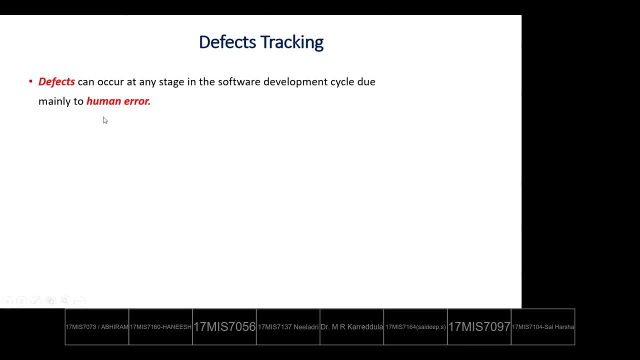 That's why. That's why humans are doing mistakes: Because of poor understandings of requirements. It's not easy to predict the client mind, What the client is expecting in terms of a solution, In terms of a product. So it's not easy. 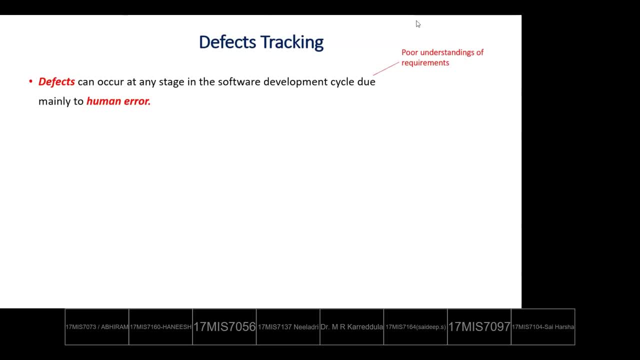 Because the client is going to define everything in terms of English like language. So humans makes mistakes called defects. A defect is anything that is wrong with the application that causes it to not meet the customer's requirements. Why we are not able to meet the customer requirements. 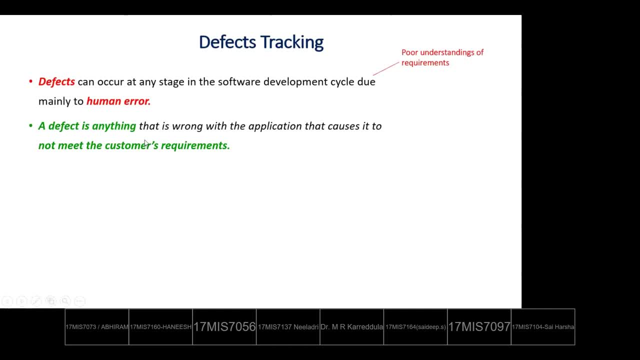 Defect is anything In the project schedule from day one to day n Anything So: the supply of human resources, The supply of papers, The supply of erasers, The supply of various other materials, So like a keyboard, Mouse, Internet facilities, 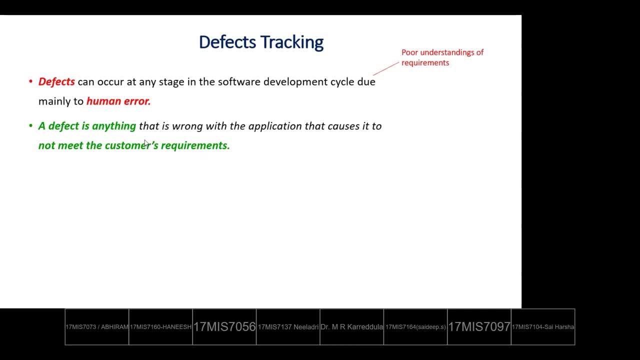 Except anything, Anything is considered as a defect in the project development. So for our understanding sake. So here we discussed poor understandings. So why poor understanding? Because of global language, English language. So that's why we are not meeting: Because of poor understandings. 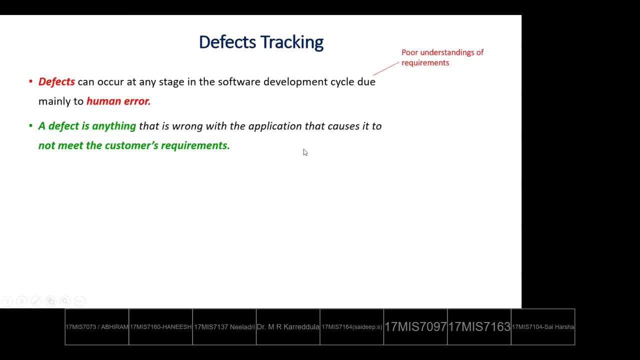 So here client will use English like language. So we convey one thing in many ways. For understanding sake I am giving this information, So we will provide some information, Good or not bad, So both will give in one way same meaning, If someone ask you. 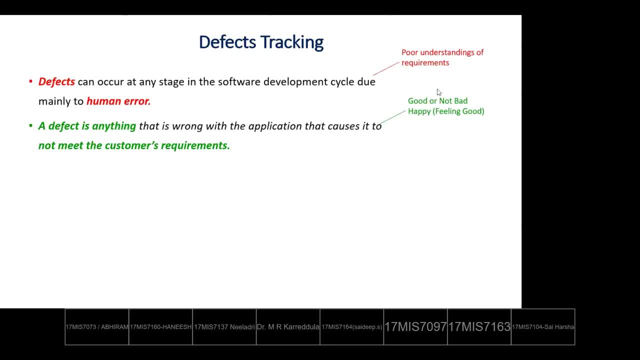 How are you? So? in one way we will use the word good Sometimes we will use not bad, So both will give same or similar kind of meaning. So here, if you see happy, I am very happy, I am very good. So that is giving a feeling good. 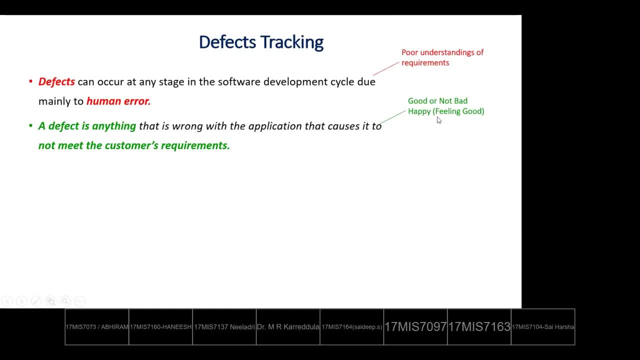 So, like this way, One thing may be conveyed in many ways, But depends on the understandings of the requirements by the various developers who are involved, The various designers who are involved, The various test engineers who are involved, Because we are developing based on the requirements, specification. 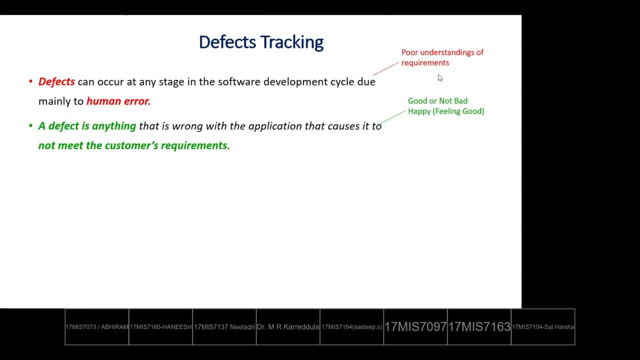 That is SRS. The test engineers will test based on SRS. The deployment engineers will deploy based on the requirements specifications only. So here we will use this SRS document for everything: To analyze the problem, To design the solution, To implement the solution. 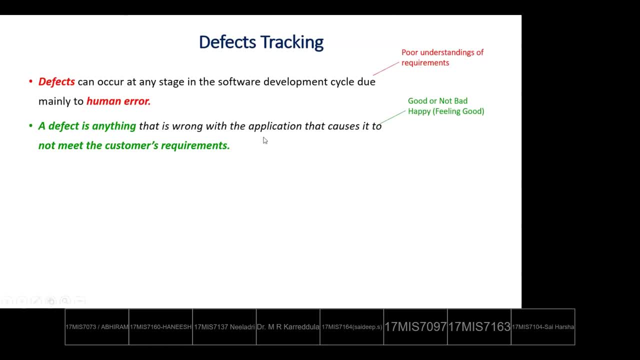 To test the solution, To deploy the product, Everything we will use SRS. So this SRS is key role. It is playing a key role in software development. So we need to understand this SRS completely. Then only we can easily finish the product. 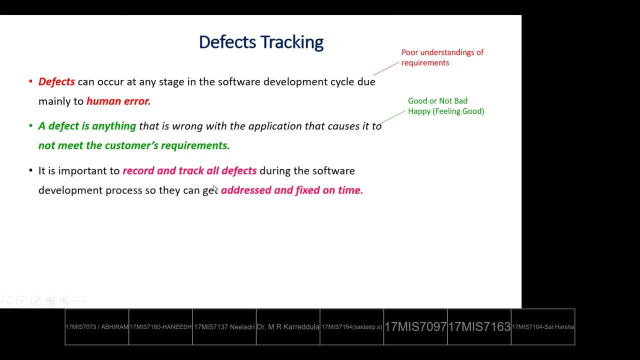 So it is important to record and track all defects. So defect is anything. So we need to record why defects are occurred, What is the damage percentage on the remaining requirements. So when it was happened, What is the status of the defect? Like this way, we need to record the defect status. 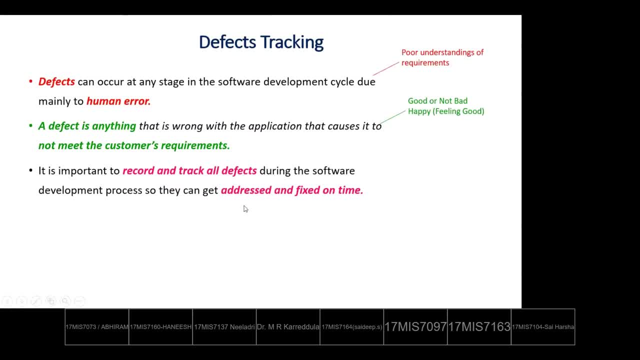 During the software development process So they can get addressed and fixed on time. So we need to fix the defect, We need to fix the defect. A good defect management system can help project managers achieve successful product development, So good defect management system is required. 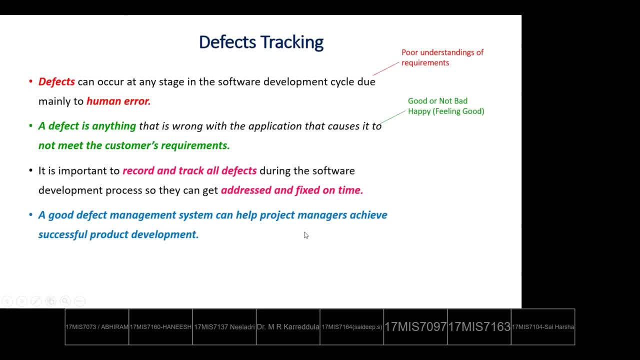 Which is useful to project managers In order to develop the product on time And deliver on time. So that is it. This good defect management system will be useful to test Q&Q, Quantitative and qualitative analysis of the whole product. Quantitative nature and qualitative nature of the whole product. 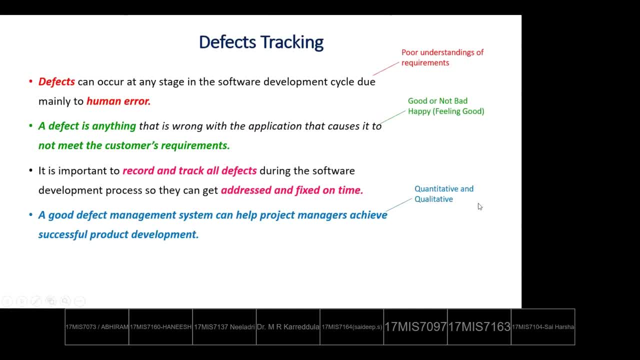 So we are tracking the defects In order to test whether it is having quantitative- That is nothing but the various functionalities defined in requirements document And their quality Are achieving or not. In order to do that, We will find the defects And closing the defects. 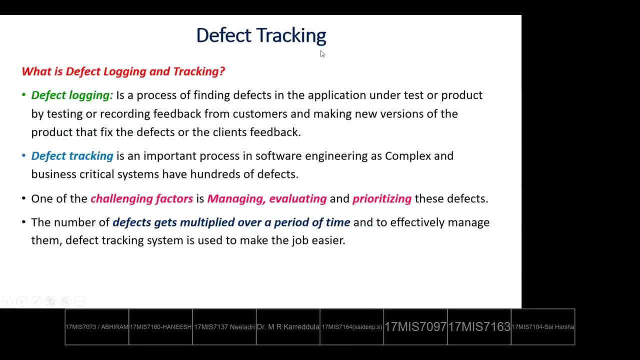 So we will see. So defect tracking: What is defect logging? and tracking While identifying the defects, So when it was identified. So defect logging is a process of finding defects in the application under test or product. So process of finding defects in the application under test or product. 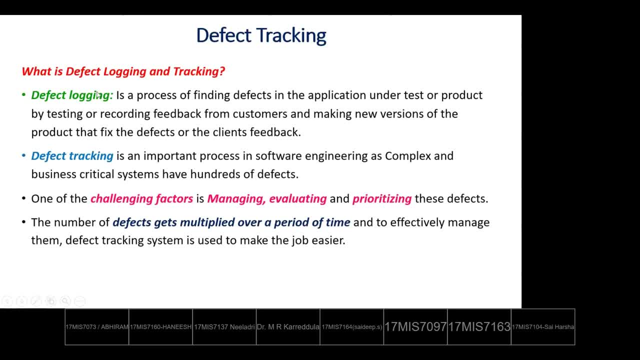 So during testing only we can identify the defects By testing Or recording feedback from the device, Or recording feedback from customers And making new versions of the product That fix the defects of the clients. So after fixing the defect We need to plan the alternate solution. 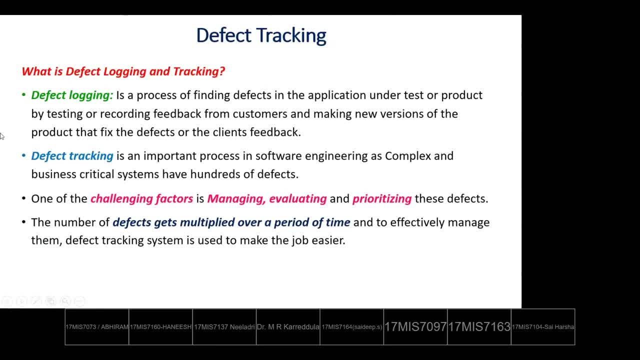 After implementing the alternate solution We need to get approval from the client. Then only we can add this solution to the actual product development. Defect tracking is an important process in software engineering, As complex and business critical systems have hundreds of defects, So sometimes these defects may be. 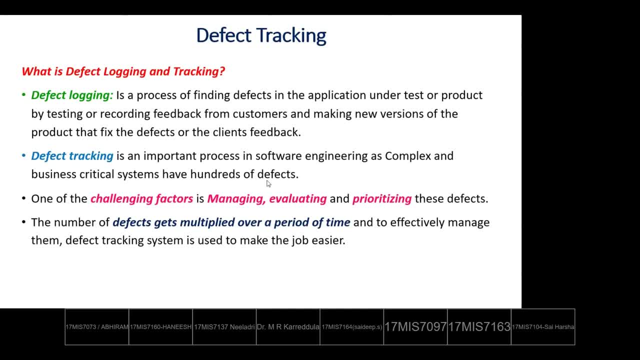 Identified in terms of thousands. Sometimes, if it is a large scale project During development, we can identify thousands of defects. So one of the challenging factors is managing the defects, Evaluating the defects And prioritizing these defects. So here we won't pay attention to all the defects. 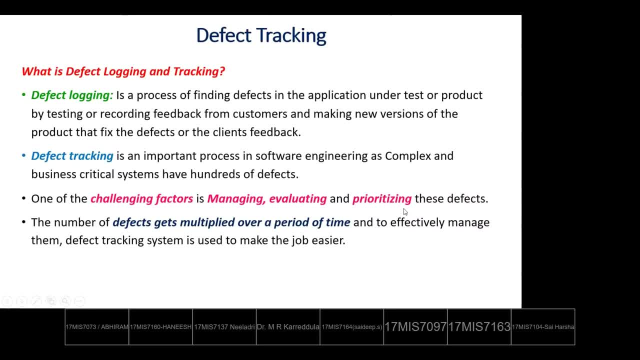 We will prioritize, So, as we know that, how the product development starts and finishes, So in terms of releases, Or in terms of various projects, Or in terms of various versions, So we will focus majorly Which defects need to address immediately. 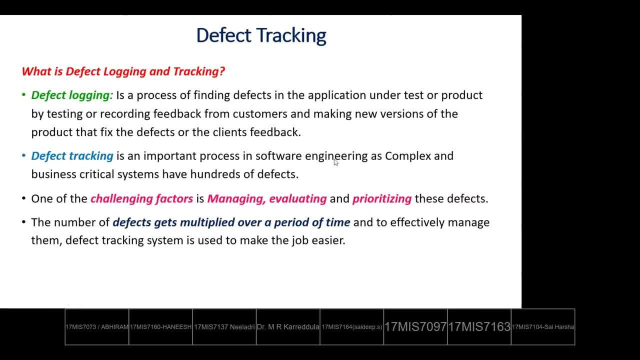 Those defects are identified and addressed. I mean planning the alternate solution And implement the alternate solution And adding to the existing, That is, integrating with the existing. So here we are majorly focusing on Which defects need to address immediately. Those defects are added. 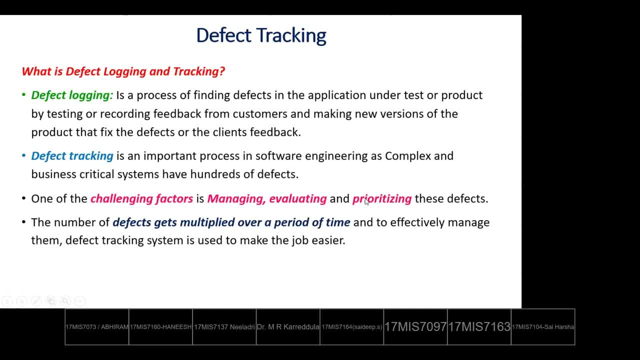 Or integrated immediately. Later we will add the remaining defects And releases as a new version. So that is a challenging task. in software development The number of defects gets multiplied over a period of time, So generally it is happening So when one defect is identified in one module. 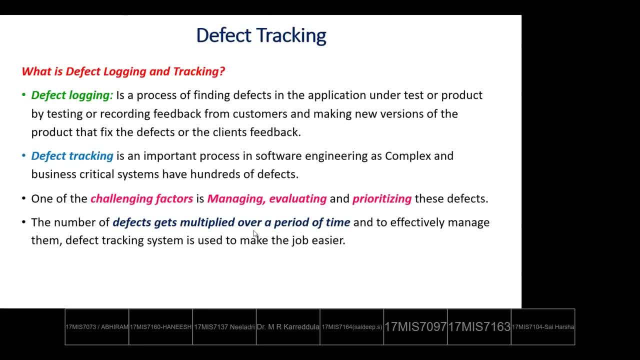 When it is integrated with other modules. So it may support, May not support. If it supports, No problem. If it doesn't support, It leads to another problem. So generally it is happening With regression testing That you studied in software engineering. 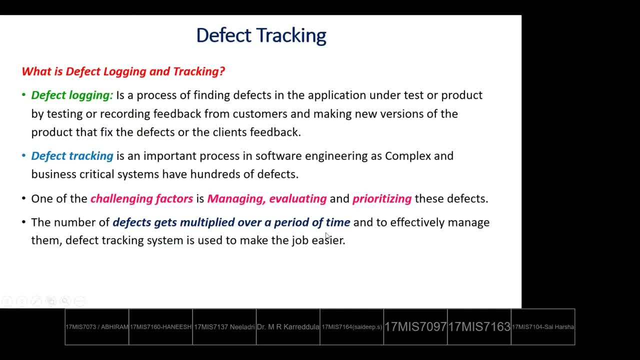 Regression testing. So what do you mean? regression testing, When we integrate two inputs, Generates a third input. What called Testing the third input Is what called regression testing. So that is generally happening In creation of data warehouse And databases. 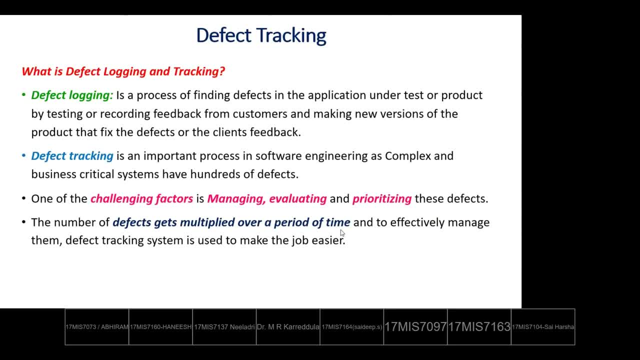 So when two inputs are Tested, Third input is generated. Testing the third input Is what called regression testing, So industry focusing on regression testing. So, in order to resolve the defects And to effectively manage them, Defect tracking system is used to make the job easier. 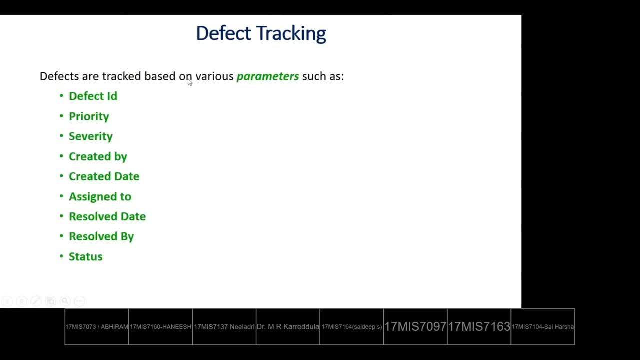 So we will see defect life cycle. So these are the different parameters are used in the defect tracking Defect ID. So we have to identify the defects And assign the number, The defect ID, In which Stage it is Identified. 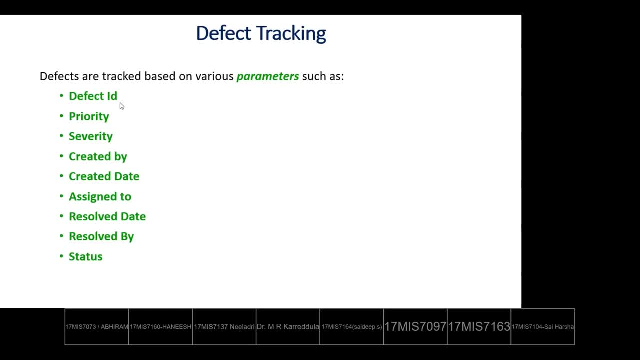 That is, analysis stage Or design stage, Implementation stage Or coding Testing stage, Etc, Etc. So if it is identified in development stage, In which model it is identified? Like this way, we need to identify, So we need to give a. 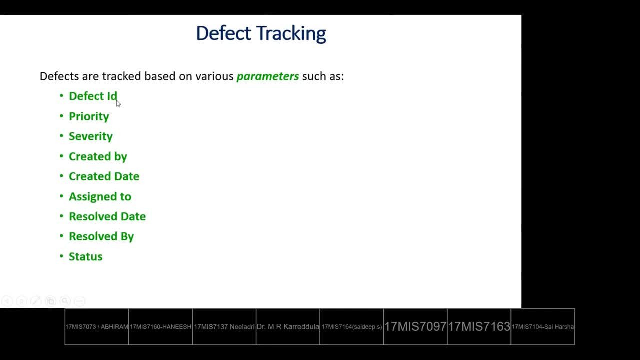 Unique Identification number For the defect And priority: The priority of the Defector, So high priority Or low priority Or medium Priority. And severity. So we need to give A unique Identification number For the defect. 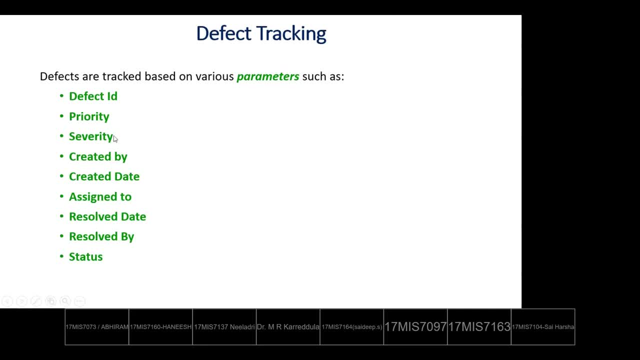 So severity Is nothing, but We need to address the Defect immediately Or Not. So that is Paying more attention Or Not Required. Created by. Created by Developer Or tester Or designer Or client. 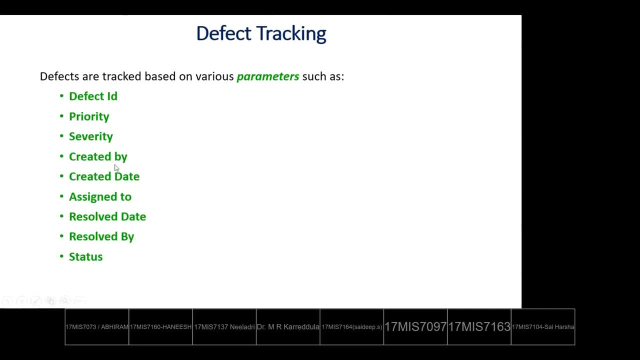 So client also sometimes Identify the defects, So it is created, Created by. So I- I hope we discussed The definitions of Error, Defect, Bug, Etc, Etc. Please go through that. So what do you mean? 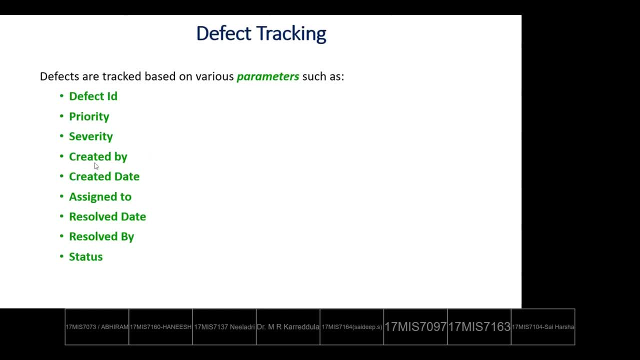 Error? What do you mean Failure? What do you mean Fault? What do you mean Defect? Okay, So Created by Whom? Analyst? A designer, A developer, A tester, A maintenance engineer Or client? 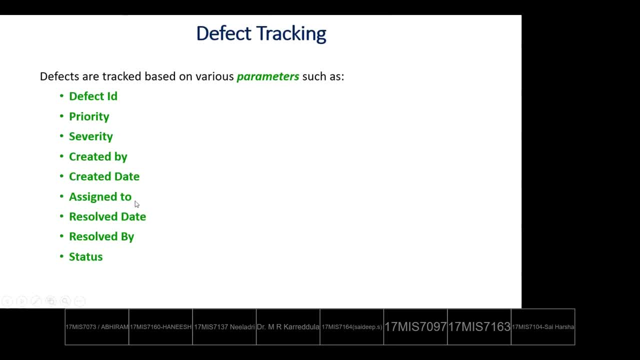 Etc. Etc Created date On what date It was Identified, Assigned to Whom? Assigned to Developer Result: Date Result By So here Result: The solution is prepared For the defect. 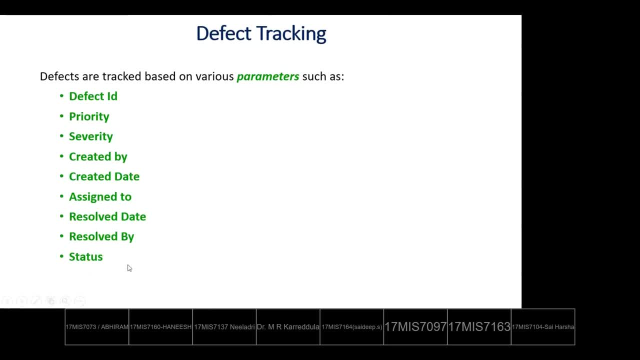 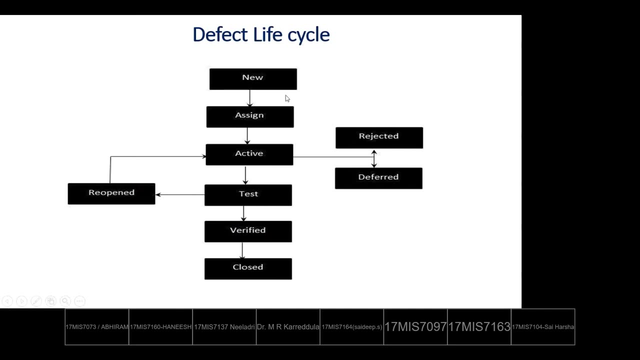 By Either Designer Or developer Or tester, Any person And status of the Defect During the Project Development. So Various parameters Are identified And This is Recorded. Now We'll see. 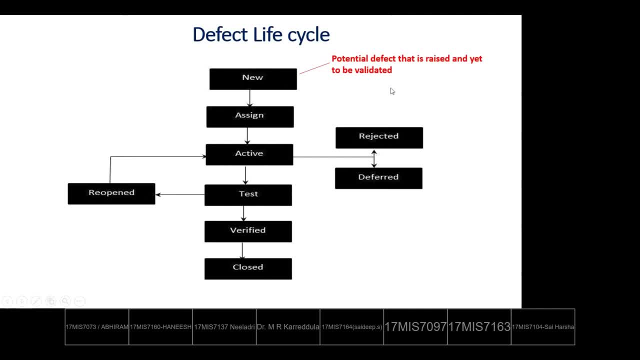 Defect Life cycle To be Validated. So Once The defect Is Identified By Developer, We Cannot Say It's A defect. We Need To Get Approved Whether. 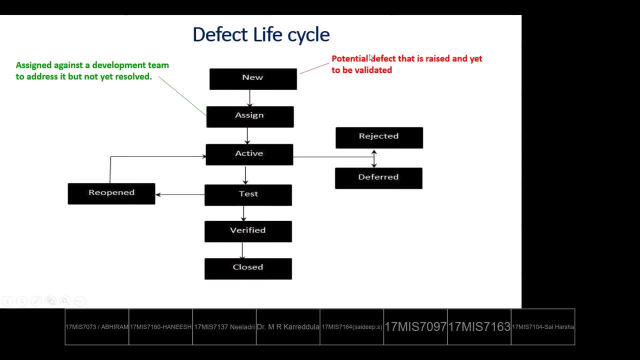 It Is A defect Or Not. We Need To Finalize, So We Need To Give To The Development Team. So Development Team In Themselves Identified. 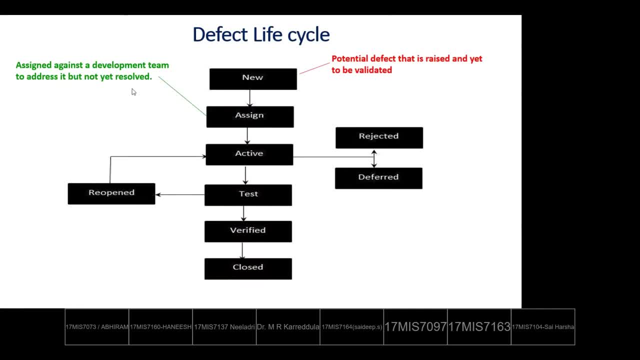 So Themselves Will Identify One Person And Assign The Defect To That Particular Person. So, After Assigning, This Particular Team Will Resolve The. 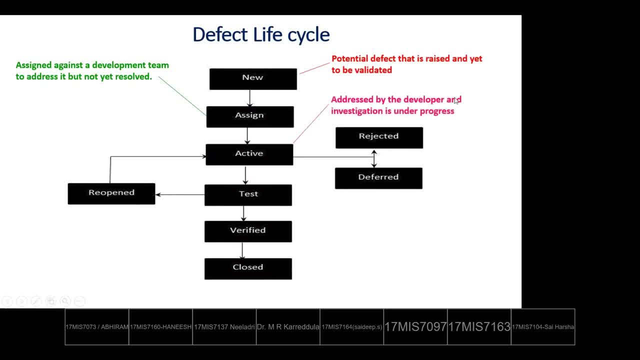 Defect And Notice The Status: Status In Terms Of Either Rejected Or Deferred. So Deferred Is Nothing, But We Can, So Best Example For This: 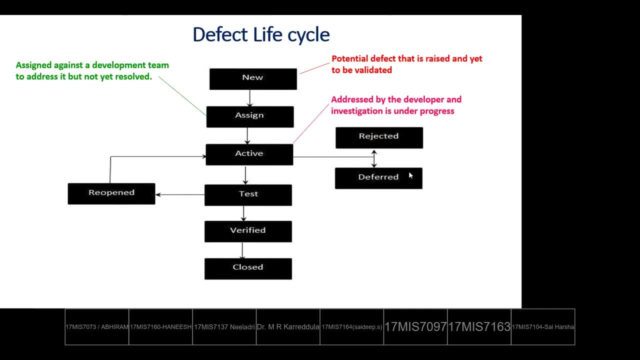 Is The Cell Phone. Companies Are Launching Various Products Or Various Versions Of Their Products. Take Samsung Weibo, Etc. Etc. So Every Time They 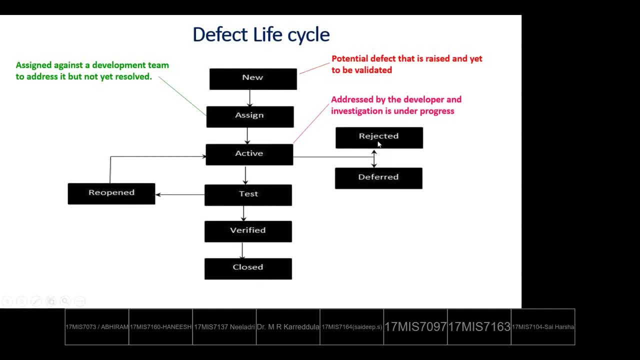 Have A Defect For Future Versions In Future Versions Are Rejected. So, Due To Various Problems, This Defect May Be Rejected. So Someone Says: 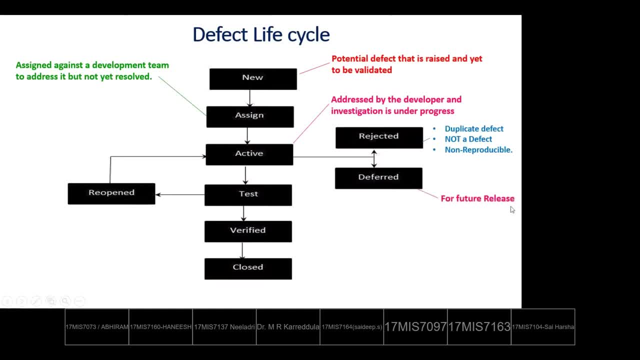 It Is A Defect. That Is S Defect In Future Versions, Then Testing Defect Is Fixed And Ready For Testing. So After Fix Fixing: 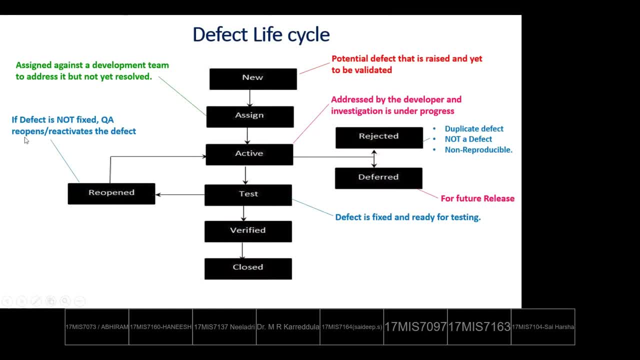 The Defect And Planning The Alternate Solution After Implementation: Again Go Defect. that is retested and that test has been verified by quality assurance team. So different people: the analyst, designer, developers, testing, quality assurance engineers. 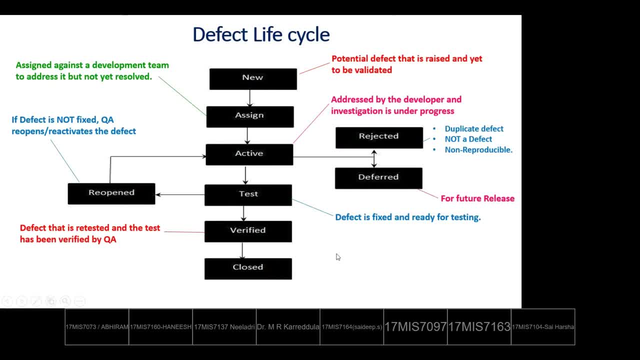 So like this way, different people are testing or working on the defects and finally closed. Final state of the defect. that can be closed after the QA testing, after quality analyst testing the whole defect. If he confirms it is not a defect or identified solution for the defect, they will close. 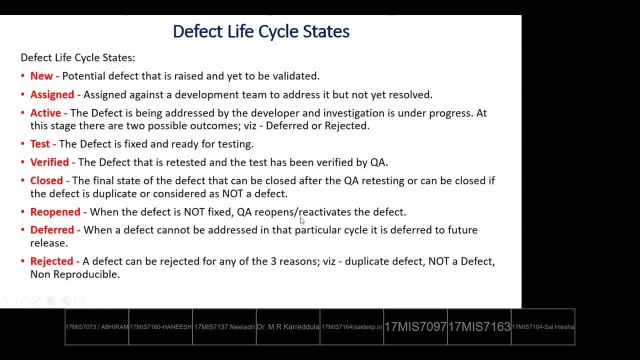 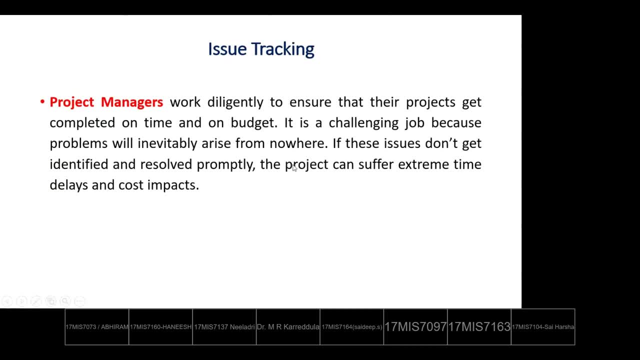 The defect. So these are the stages of the life cycle of defect. So issue tracking, now issue. project managers work diligently to ensure that their projects get completed on time and on budget. So as a responsible project manager, I have to deliver the solution to the client by the 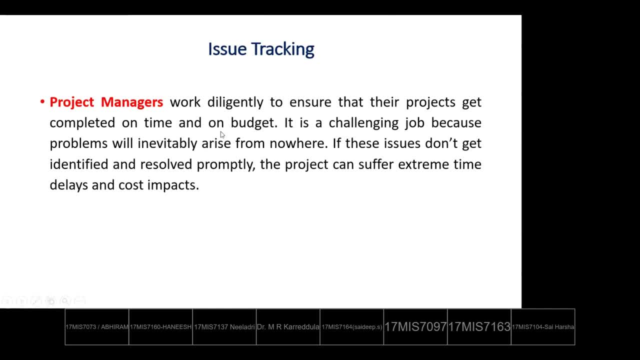 given deadline and within the budget. So this is the key factor that we have to keep in mind as a project manager. So it is a challenging task. It is a challenging job because problems will inevitably arise from now here. So at any stage the defects are identified or issues are identified, from day one to day. 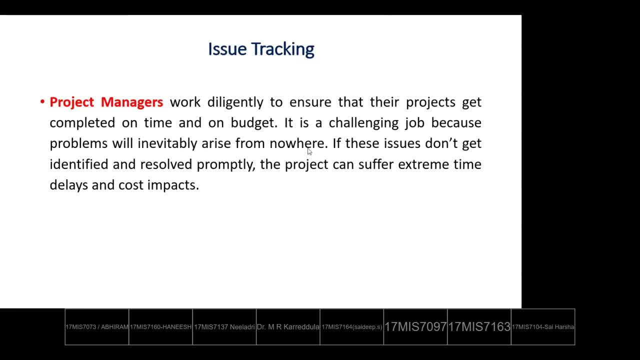 end. So we need to resolve all those defects, issues, bugs, errors and so on. So many resources problems, So we need to find a solution. We need to deliver on time within the specified budget. only If these issues do not get identified and resolved promptly, the project can suffer. 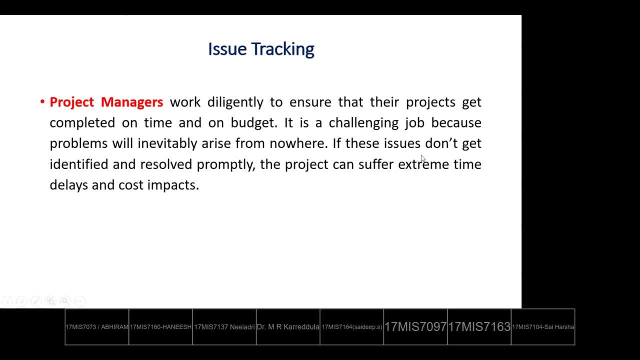 extreme time delays and cost impacts. Okay, So if the delay and cost the difference between the cost, that is, a planned or estimation cost and implemented cost, if there is a low difference, if the difference is less, they can accept it. if it is more, 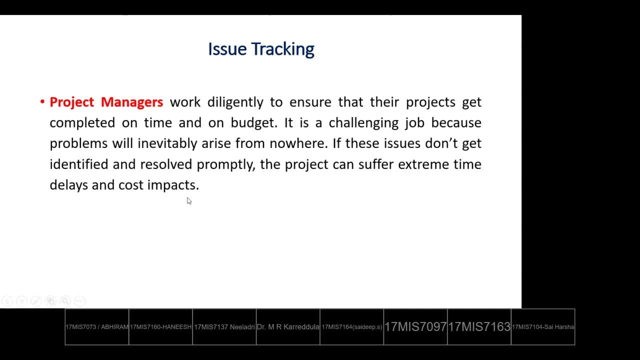 So if it is taking more time, if the cost is increasing. So sometimes as a project manager I need to answer for everything why it is delaying. So, like this, issues tracking in that process, issues tracking, Issue tracking system is very important. 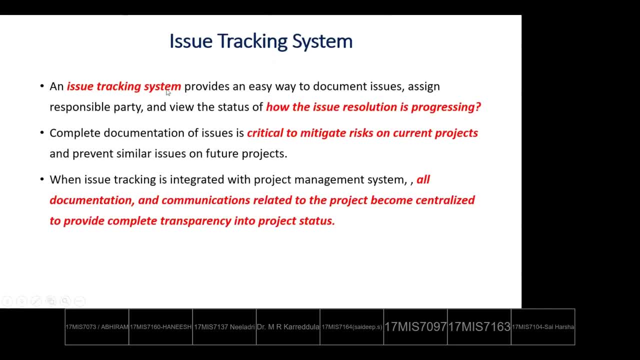 Okay. Issue tracking is developed in order to track the issues, and issue tracking system provides an easy way to document issues, assign responsible party and view the status of how the issue resolution is progressing. Responsible party means so that is, responsible developers or test engineers or who are involved. 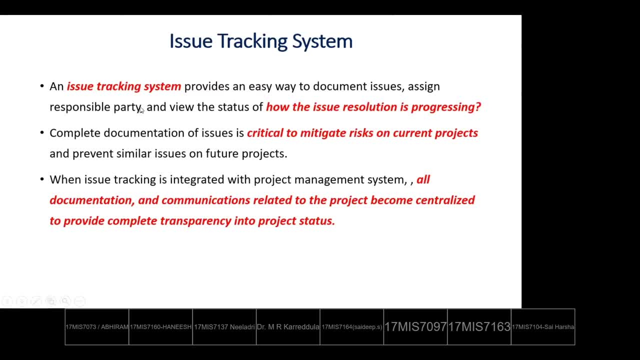 in that development. So identify the responsible party who will take the initiation to solve or find the solution for the issues. Complete documentation of issues is critical to mitigate risks on current projects. mitigation of risks: So various risks are identified, like technology risks, product size risks, business risks. 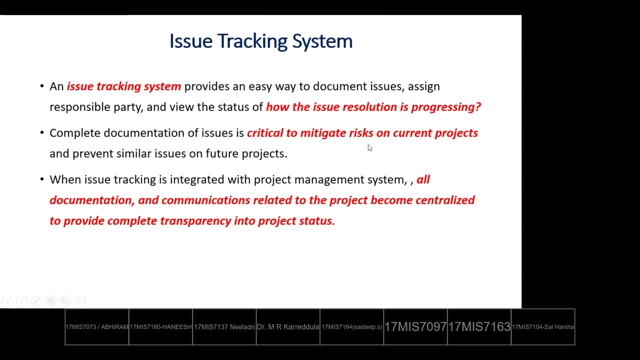 environmental risks, et cetera, et cetera. risks are identified. So how to mitigate those risks? when issue tracking is integrated with project management system or documentation, So when this is So actually the different team is working on this, Okay. 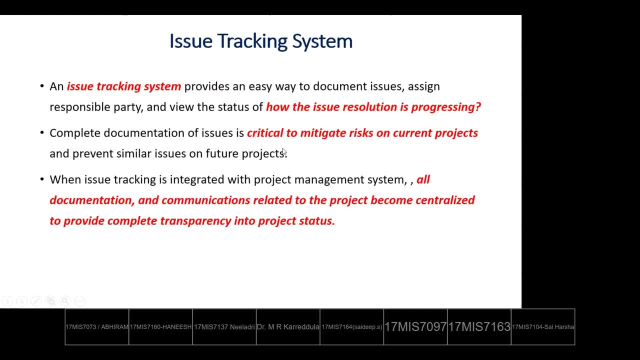 So when it is integrated with the project management system, all documentation and communication related to the project become centralized to provide complete transparency into project status. Actually, independent team or individual team is working on these issues. So if it is integrated with project management system, project management will know all the 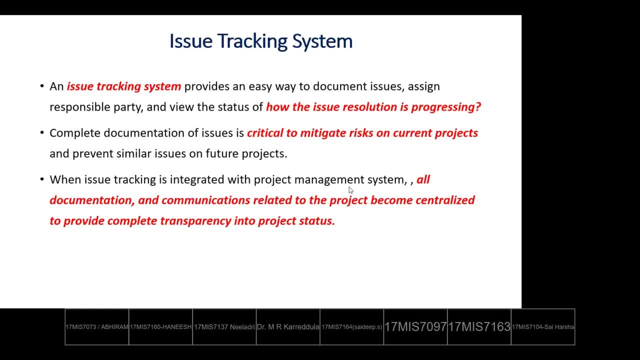 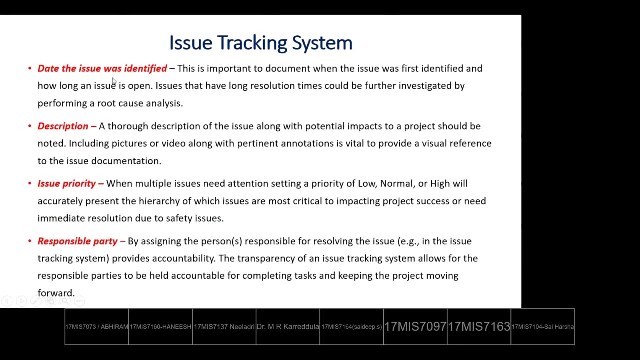 issues and the status of the issues and defects. Then we can assess the progress of the project project. So these are the various parameters: date the issue was identified like defects, So on what date it is identified. So this is important to document when the issue was first identified and how long an 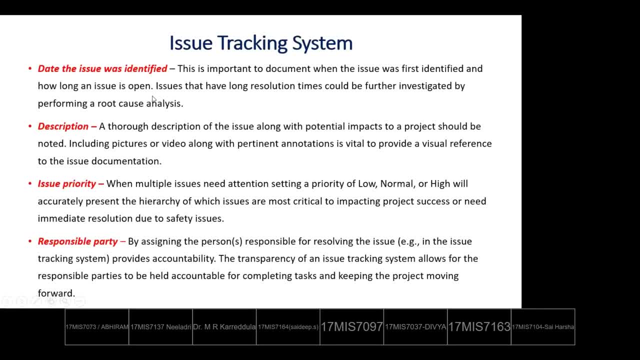 issue is open, So that is the closing time of the issue. Issues that have long resolution times could be further investigated by performing a root cause analysis. Root cause is why the issue is happening Like failure, Why the issue is happening Failure or fault. 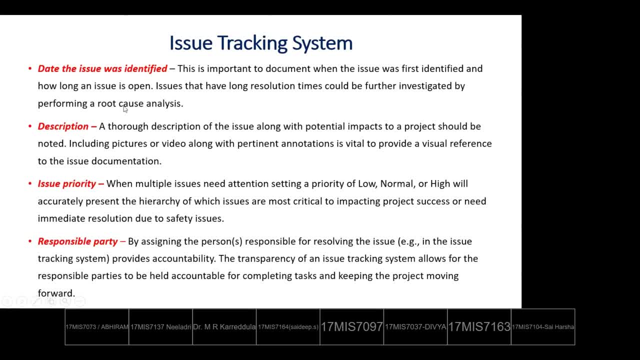 Not the error, Failure or fault, Finding the root causes why the issue is happening in the product development and description of the issue. A thorough description of the issue along with potential impacts to a project should be noted. including pictures or video along with pertinent annotations, is vital to provide. 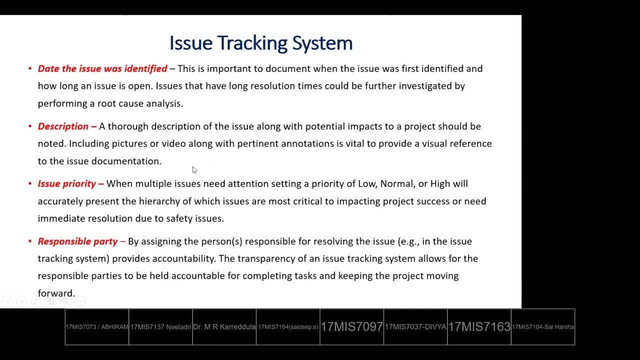 a visual reference to the issue documentation, So the complete description about the issues where the issues occurred in a module or submodule or sub-submodule and so on. Issue priority: So we are giving the priority for the issues when multiple issues need attention setting. 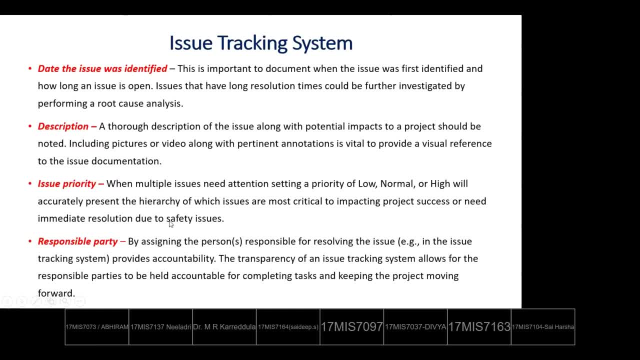 a priority of low, normal or high will accurately present the hierarchy of which issues are most critical to impacting project success or need immediate resolution due to safety issues. So here we are giving priority: low, normal, high. So high issues are immediately addressed. 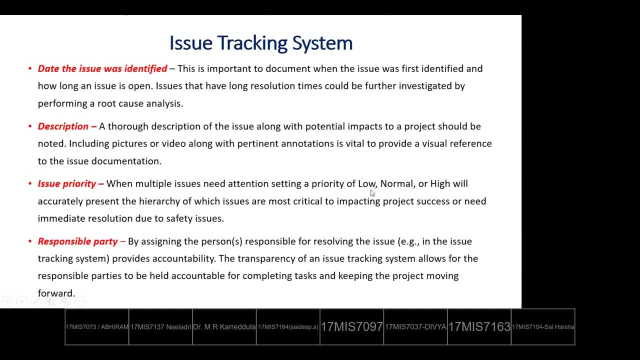 So low. issues are High Later addressed, That is, in terms of next version or next release. Responsible party By assigning the persons. So identifying the responsible persons Responsible for resolving the issue, Provides accountability, The transparency of the issue, the issue track, Complete tasks and keeping the project moving. 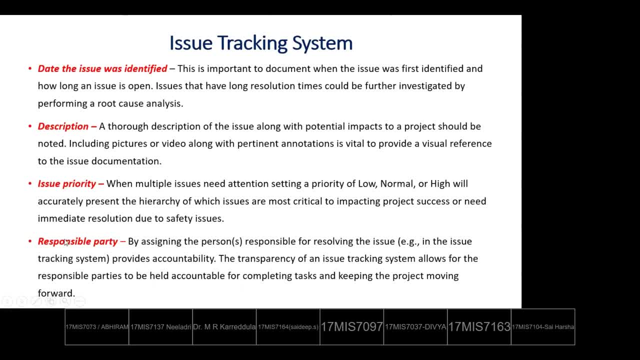 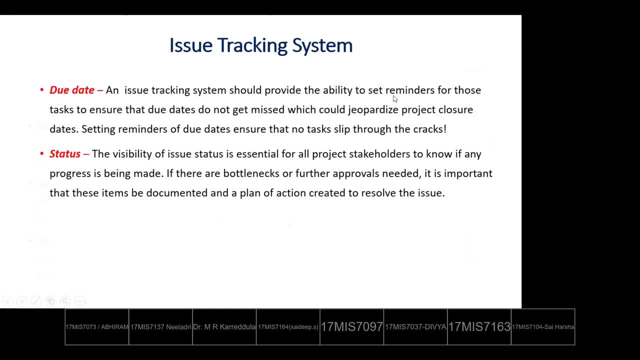 forward. So like we again need to identify the various parameters- Facility and contract management parameters- in issue tracking system, due date: an issue tracking system should provide the ability to set reminders, reminders, reminders about target dates, target dates: when should be it is open. when should we have to close? when we have to close for those tasks to ensure. 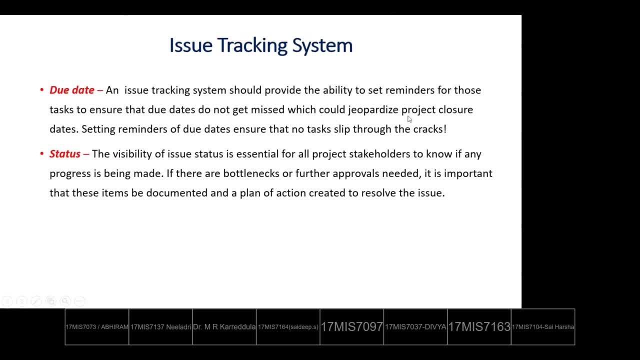 the due dates do not get missed, which could jeopardize project closer dates. setting reminders of due dates ensure that no task slip through the tracks, that is, without violating or without overlapping the schedule. how to overcome these issues are addressed then. status, so the visibility of issue. status, so what is the current status of the issue and what day it was identified? 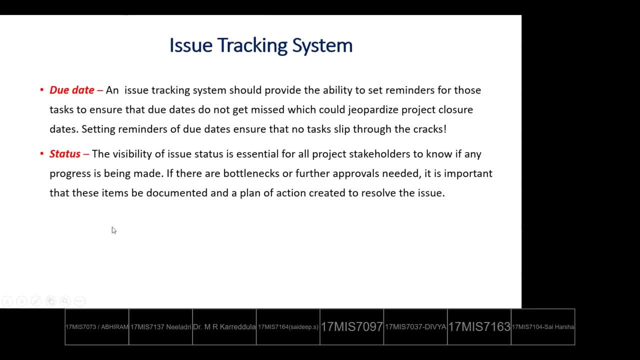 and what is the current status of the issue? who is working on this issue? what is the status? like this, we will collect a report from the people to know if any progress is being made, if there are bottlenecks or further approvals needed. it is important to but that these items be documented and a plan, a plan of action. 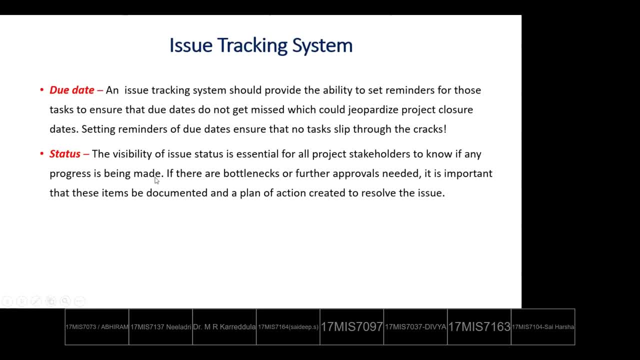 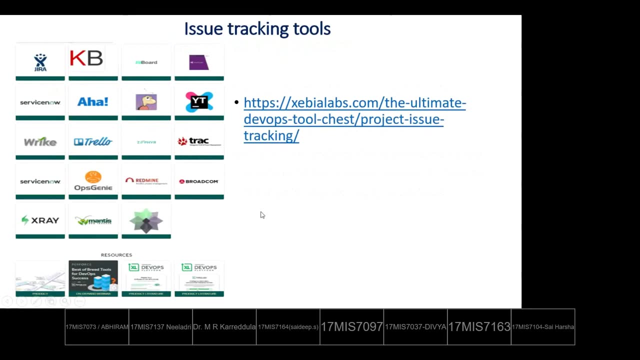 created to resolve the issue, so we need to plan alternate solution if it is not overcome how to overcome the issues. so, like this way, we need to identify the various issues and issue tracking system, and these are the various issue tracking tools are available in the system. 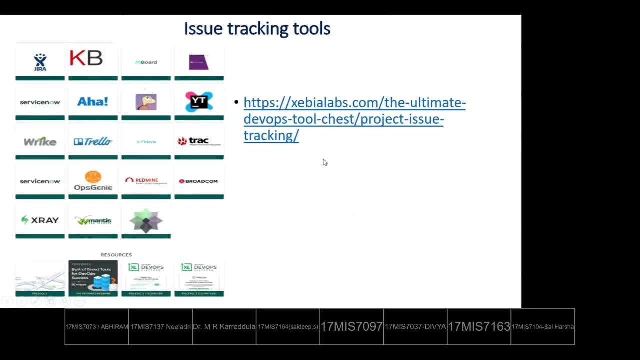 available today in the market. so this is the link so you can verify the various issue tracking system. as a project manager, i am the responsible from day one to day n until delivering the product. that is nothing but deploying the product at the client end. so i am the responsible person. so in that process, in software development, from day one to day,